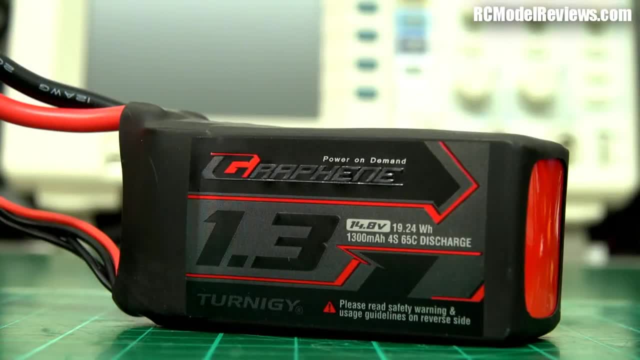 as a precursor to the reviews of the Turnigy Graphene batteries, because I want to talk about some really fundamental issues such as internal resistance. But until I've explained what resistance is and what voltage is and what current flow is and what power is, it wouldn't 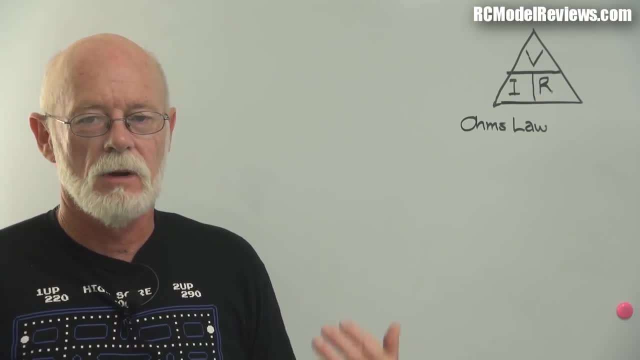 be much use doing that video. So I'm going to assume that everybody knows nothing, which in my case is pretty close to the truth. but I'm going to lead you through the basics Now. if you already know about Ohm's Law, you might find this video very boring. so 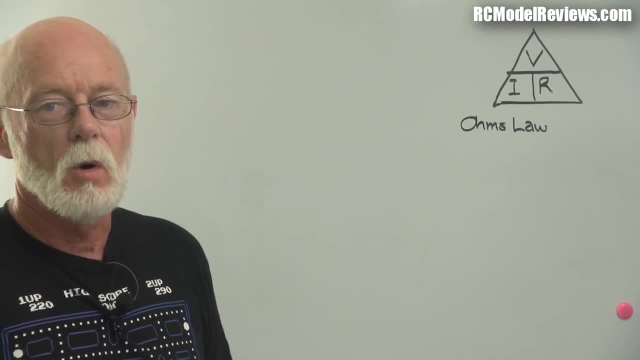 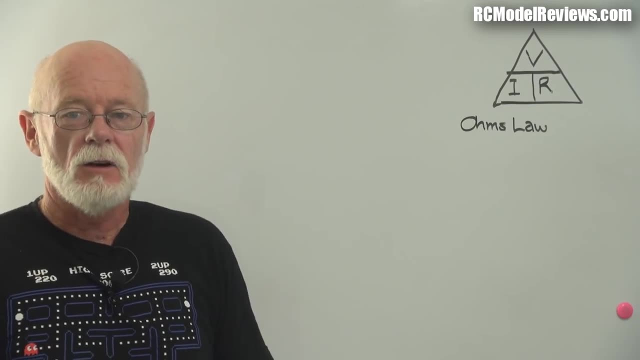 I suggest you switch over and watch something on the other channel. But if you want to be refreshed, if you want to know about Ohm's Law, stay tuned and I'll do my best to educate you Right. as far as electricity goes, we've got three main things. We've got voltage. 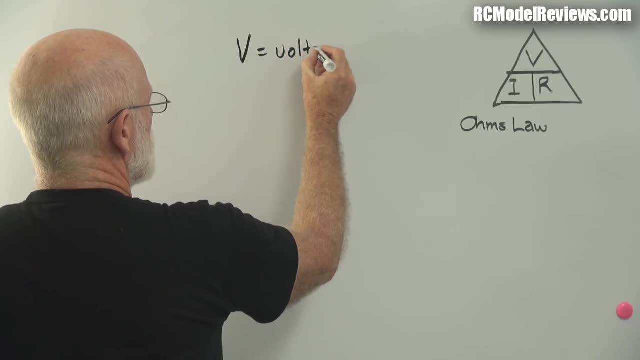 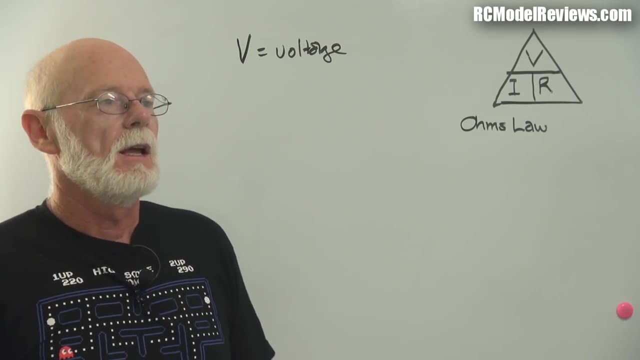 which is V equals voltage. There you go, voltage. And we know that batteries have a voltage. you know, the three-cell LiPo is 11.1 volts and the mains voltage, depending on the country you live in, can be 110 volts, 230 volts. So voltage is a measure of what we call the 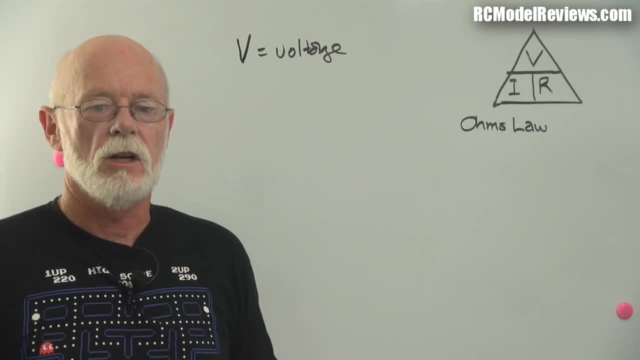 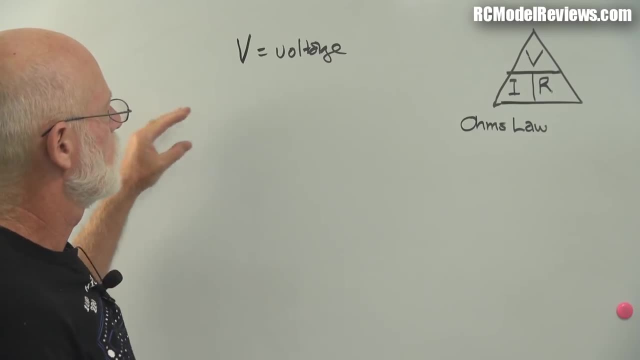 pressure. Well, analogy is the pressure of electricity. It's like water pressure. You know, when you have a water mains it might be 60 psi or whatever. That's the pressure, and the pressure is the same as the voltage. It's the voltage or the pressure that tries. 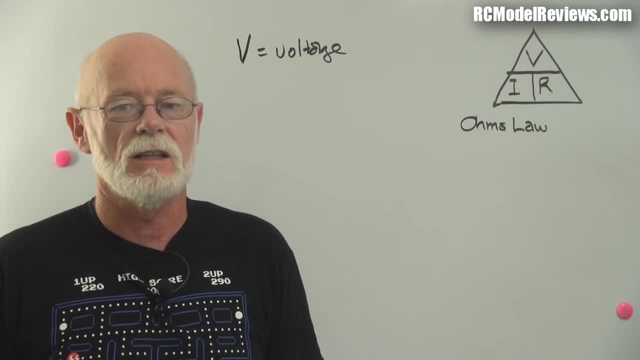 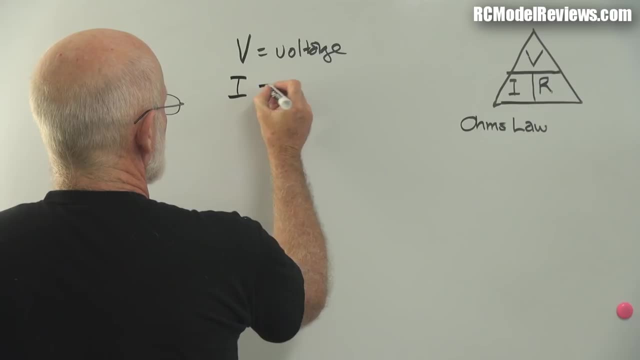 to push the electricity through the wires, through the motors, through whatever we've got connected to our battery. So it's the driving force, is the voltage. Now, the next thing is something that we call I, but it's actually the current, I suppose. 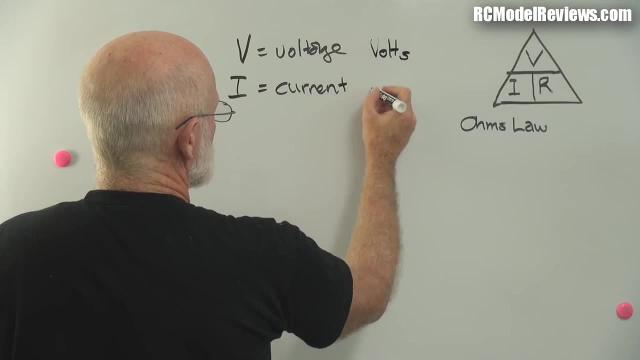 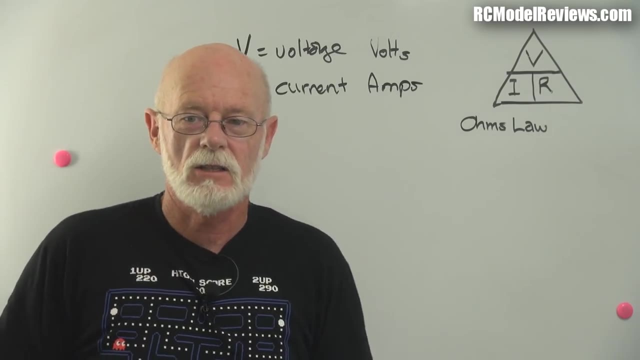 I should write: voltage is measured in volts. of course That makes a lot of sense. Current is measured in amps. There you go. Those are the measurement units. So we use the symbol I. I don't know why. I guess I should know, but I've forgotten years ago so it doesn't. 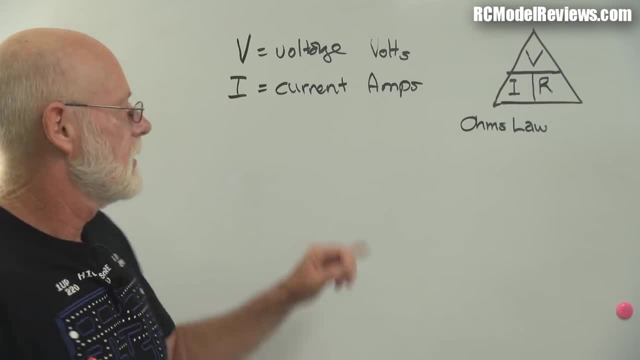 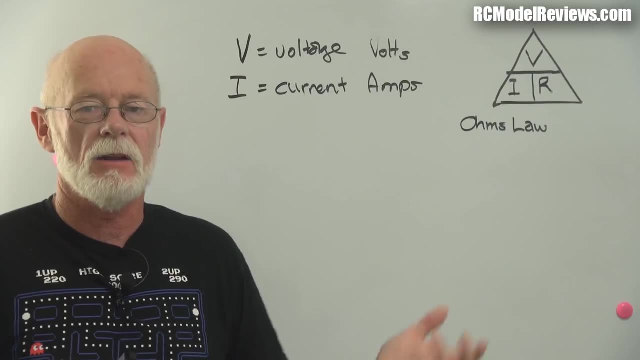 matter. But we call the current, is called I, And the current is actually relating it back to water. It's the flow, It's the amount of electrons that are actually flowing through a wire or any part of the circuit. So the voltage is the pressure, It's what's pushing things. 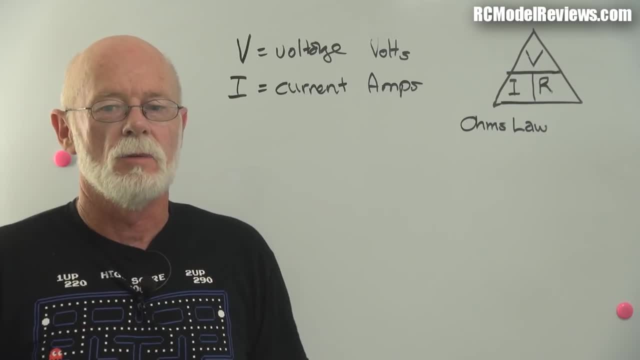 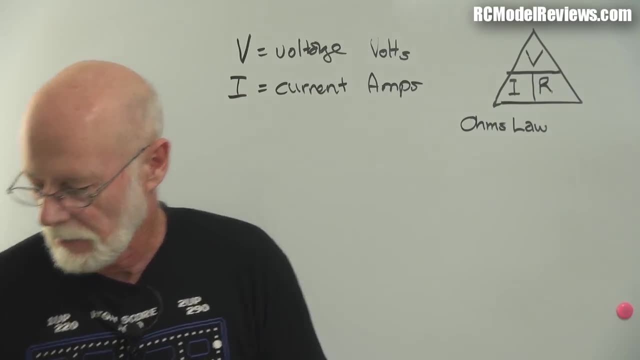 And the current is the flow. It's the actual amount of electricity or amount of electrons that are flowing through a particular part of the circuit. I've got to fly in here. I'm going to kill the bloody thing, Hang on. And the other factor involved in our circuit is: 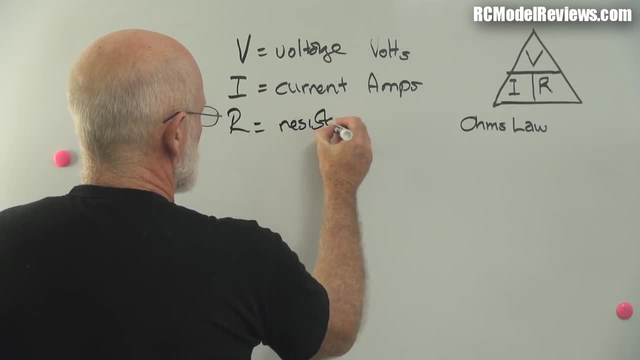 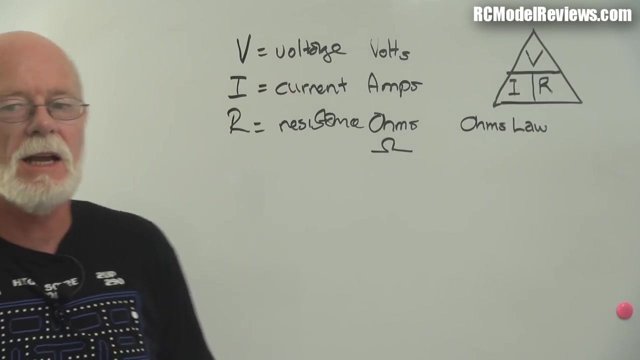 R equals resistance And that's measured in ohms. Ohms. Sometimes we use the little sigma. Was it omega? Omega, that's right. Sigma is something else. We use the omega symbol to indicate ohms. So those are the three factors that will affect how electricity 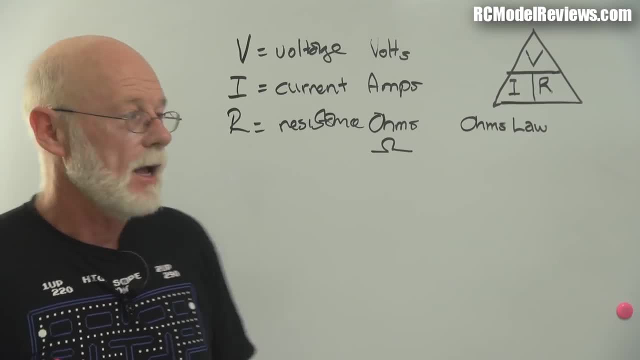 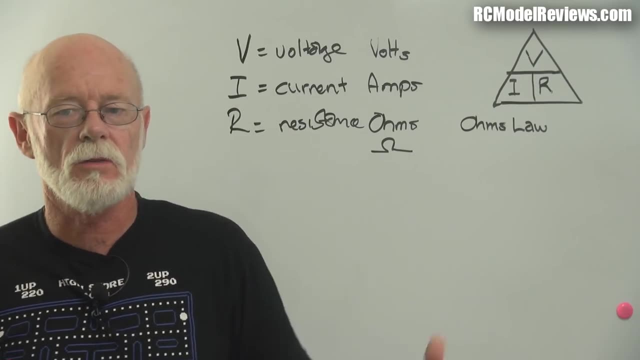 flows through a circuit, It's really not that hard In terms of water. consider R to be like the diameter of a pipe. You know small pipes. it's much harder to push a given amount of water through. So you need more power. So you need more power. So you need more power. 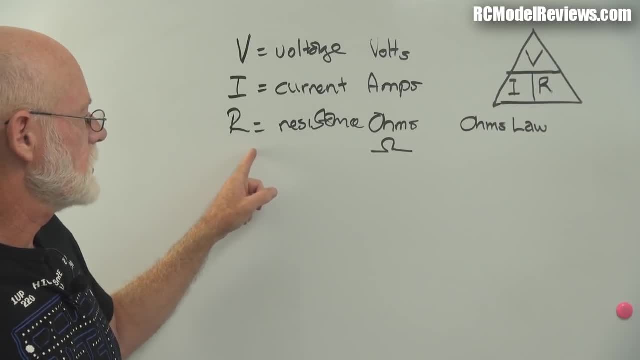 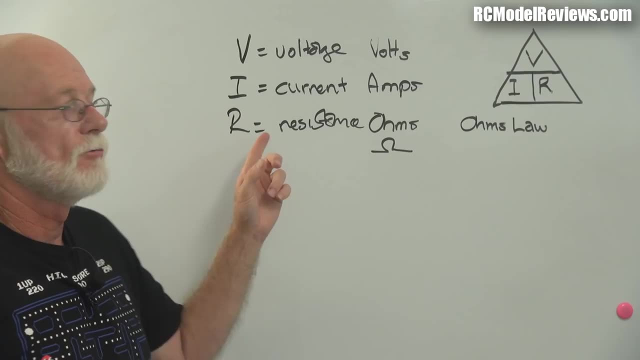 So you need more pressure, And it's the same. High resistance is like a small pipe. You need more voltage to push the current through a high resistance resistor. So these three factors are all related, And what we have over here is what I call the ohms, or everyone. 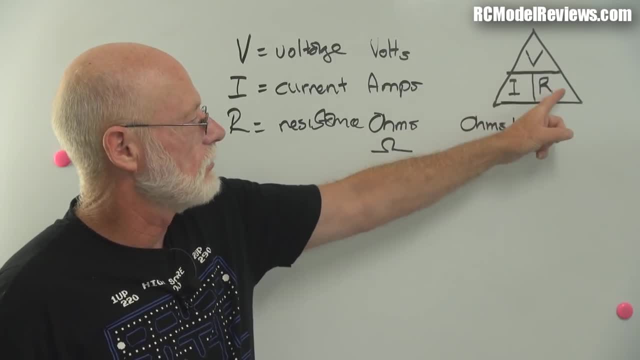 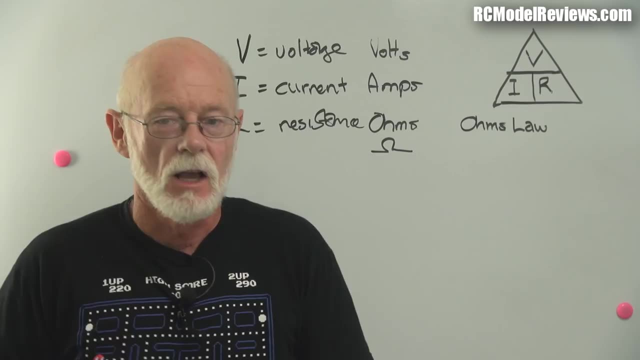 calls it the Ohm's law triangle And you can see: it's got voltage, it's got resistance and it's got current, And by drawing it in this little triangle form we can easily substitute numbers and calculate missing pieces. I'm going to draw a real simple little circuit. 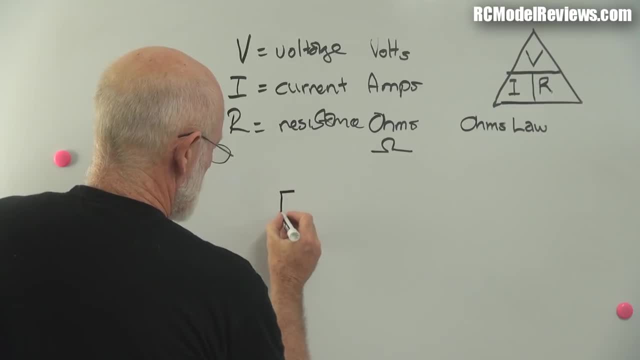 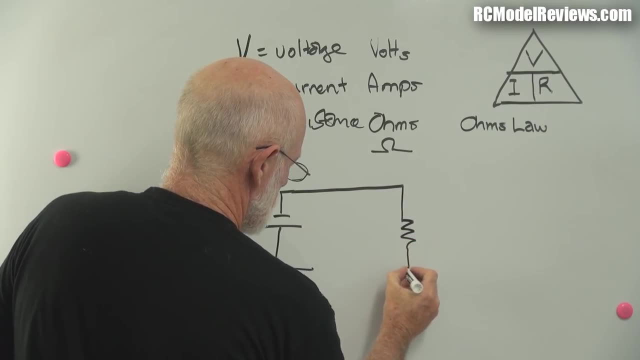 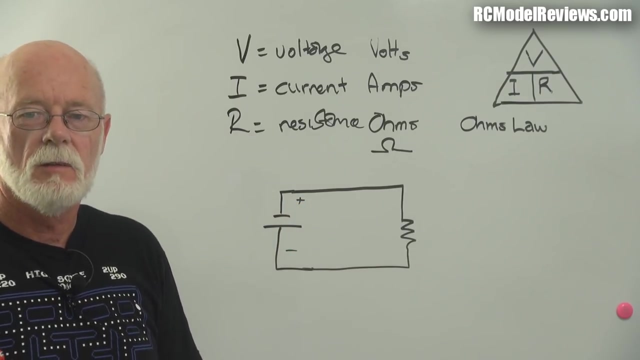 now Let's say we've got A battery And it goes through a resistor, And this is plus and this is minus, Not that it matters in this circuit, but here we go. This is a very fundamental, very basic circuit. 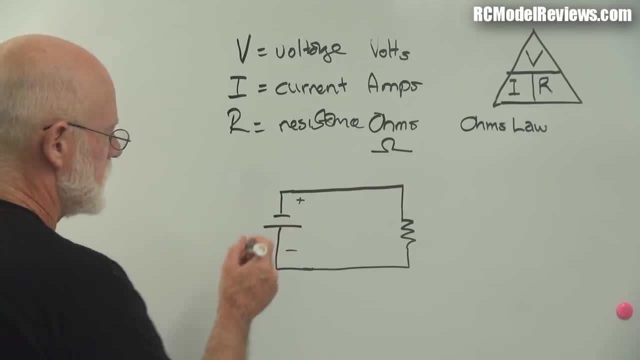 And we can do some really cool stuff. Now let's say our battery is 10 volts, because that's an easy number to work. with 10 volts, we know one of the fundamentals of our circuit. Now let's say we wanted to have 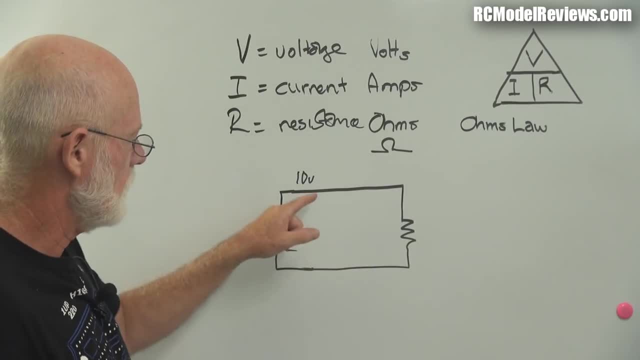 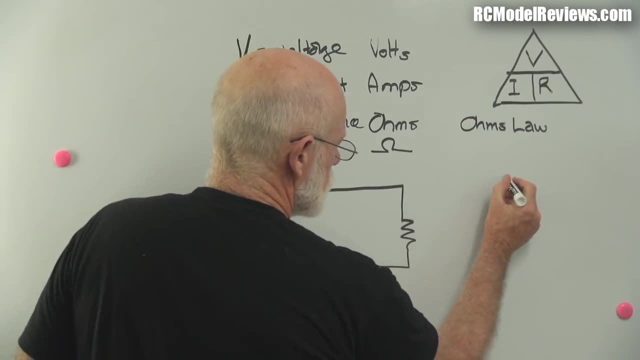 Half an amp flow through our circuit. Let's say we decided we want to take half an amp out of this 10-volt battery. What size of resistor will we need to do that? Well, we go to our Ohm's law triangle. We know our voltage. Let's draw the triangle. here We 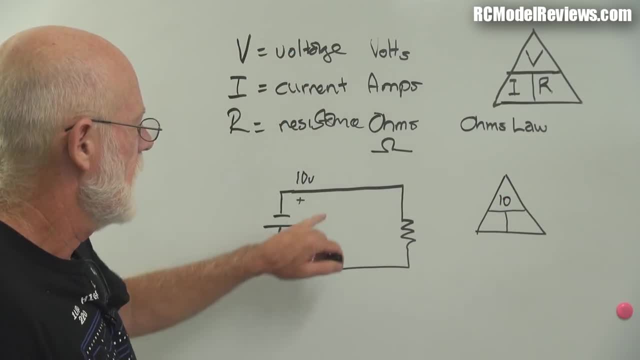 know our voltage is 10. So we can fill that bit in there Easy peasy, And we know the current we want. We want I to equal 0.5 amps. But what size resistor are we going to need to ensure that we get half an amp? We want to get half an amp. We want to get half an. 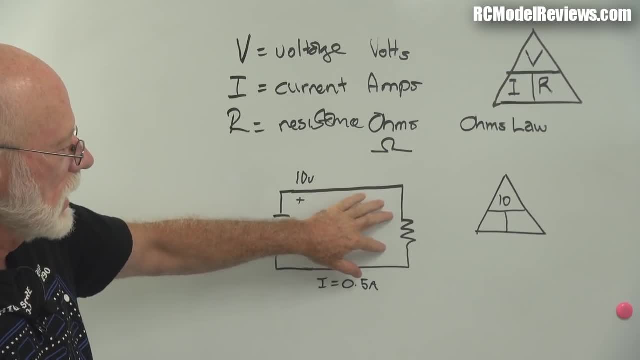 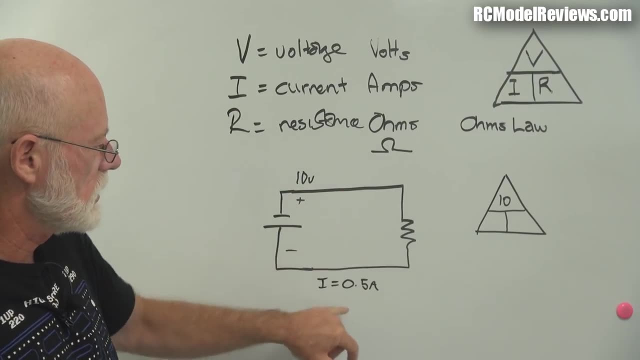 half an amp flowing because obviously the more the greater value resistor, the more it will resist the flow of electricity, so the less current will flow. we need to calculate how we're going to calculate the size of resistor that's going to give us half an amp. well, ohms law triangle comes. 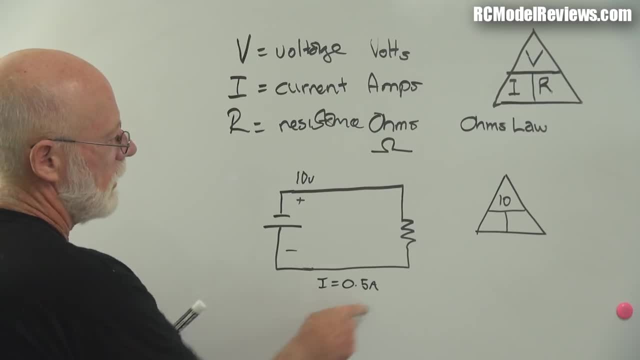 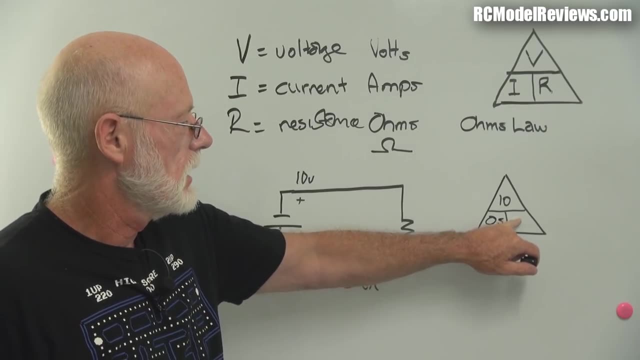 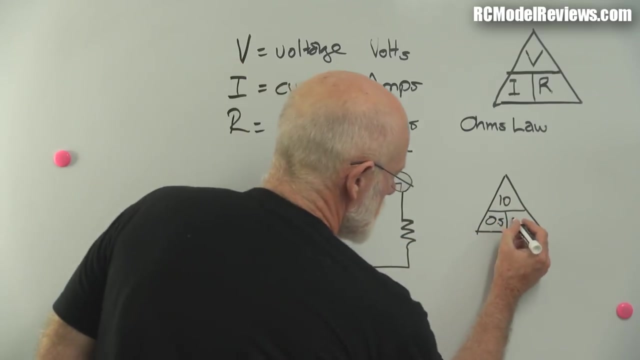 in. so we just simply we know what the i value is going to be the current. so let's just put that in there: 0.5. and now we can calculate automatically. we can see by simply: we've got a division here. we've got 10, or we've got 10 over 0.5, which is 20. so the missing number is 20. we've calculated. 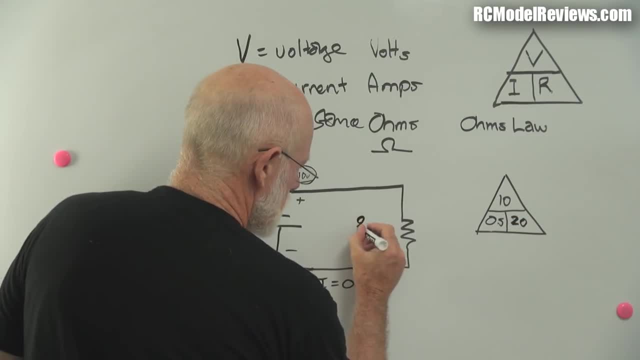 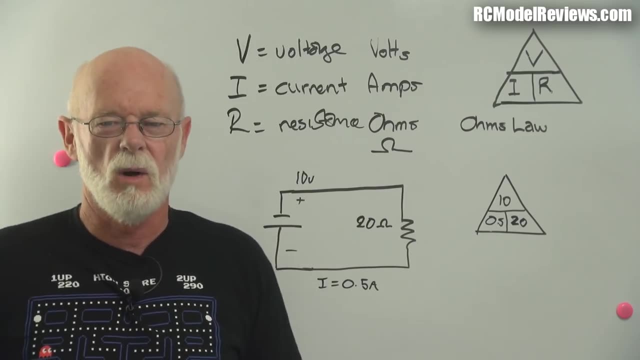 it out. so if we want half an amp to flow in here, we need a 20 ohm resistor. isn't that simple? so simple, we can calculate that basic stuff. you might be thinking right now, why would i ever want to do that? i don't give a damn about the current, but there are other aspects as well. we can. we've just 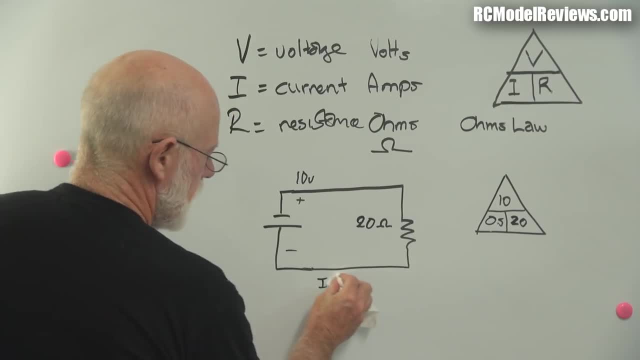 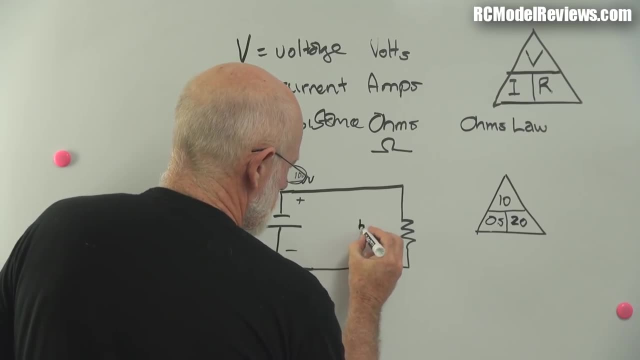 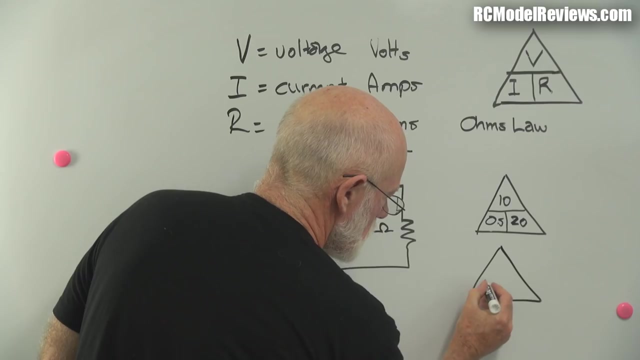 calculated the size of the resistor. what say, let's take that out. let's say we put in here a a 50 ohm resistor, so now we know the voltage. let's do another triangle, because we're using the same formulas. here we go. now we've got other unknowns. we've got a 10 volt thing, so still 10 up here. 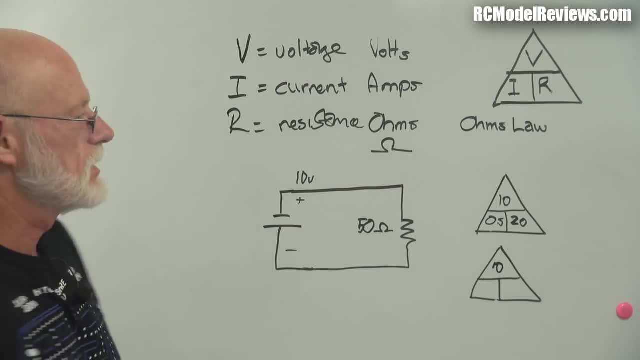 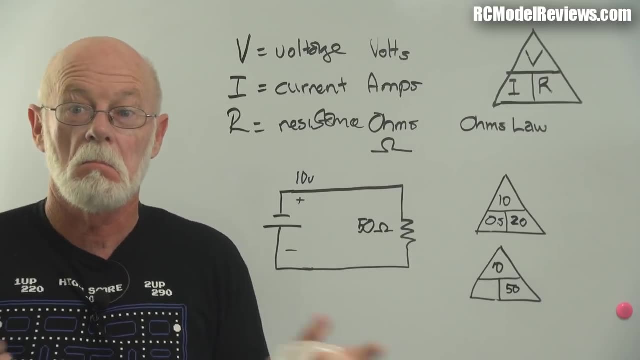 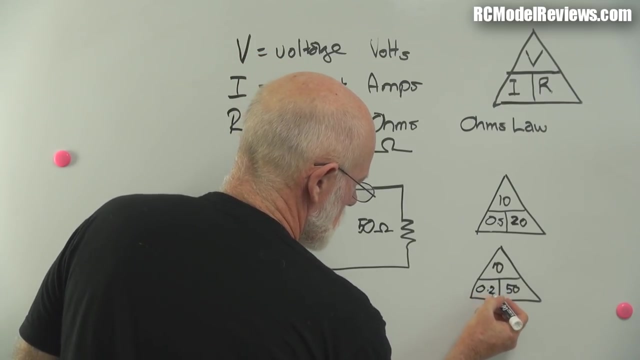 this time we know 50 ohms is the resistance, so over in here we can put 50 and we say: oh, what is 10 divided by 50? anyone got the answer? yes, it is 0.2. now, what is it 10 divided by 50? yes, it's 0.2. so now we can, and that's the i value, see i, 0.2. 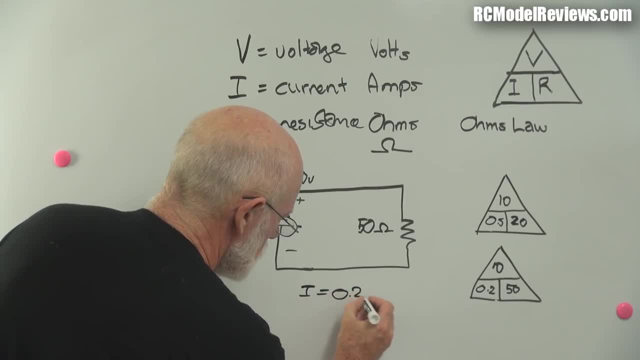 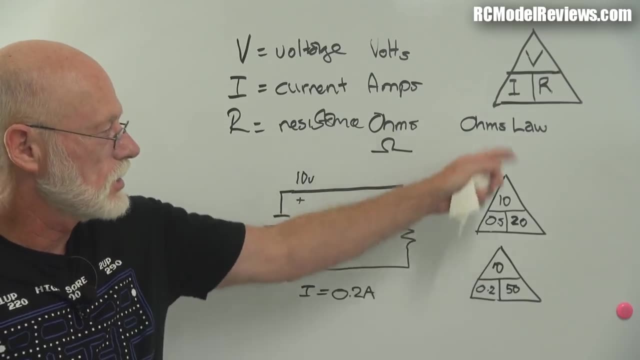 so now we can say: okay, we know that if we do that, the current will be 0.2 amps. so if we know any two of these figures, we can work out the third one by simply substituting values into our ohms law triangle. let's do the final one, because i want to show you all the options now. let's here. 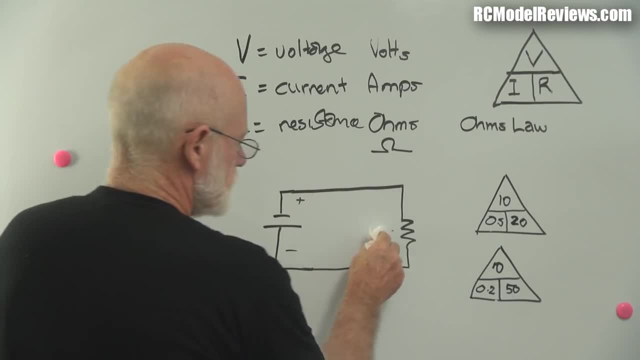 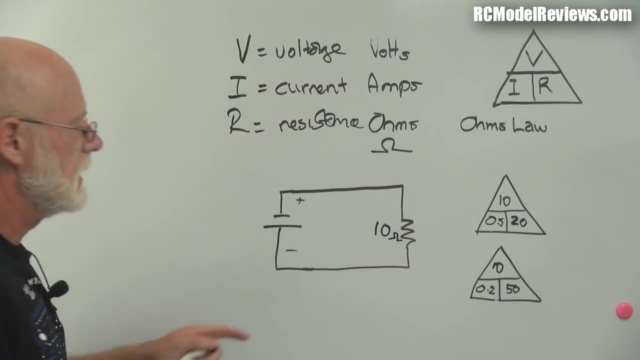 we go: let's take all these out of here. let's say we've got a 10 ohm resistor, 10 ohm resistor, and let's say we want to have two amps, two amps flowing through our circuit, so i wants to equal two. so now we've got our ohms law triangle, i'll just i'll take away this one, because 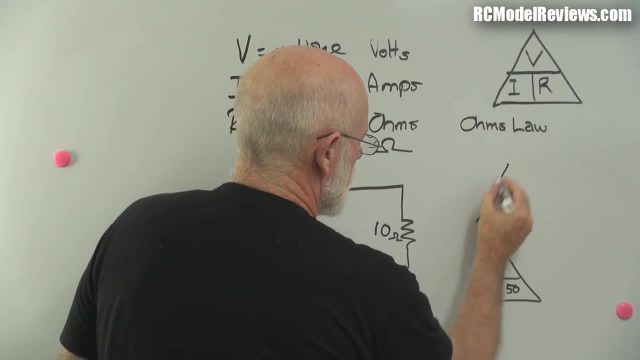 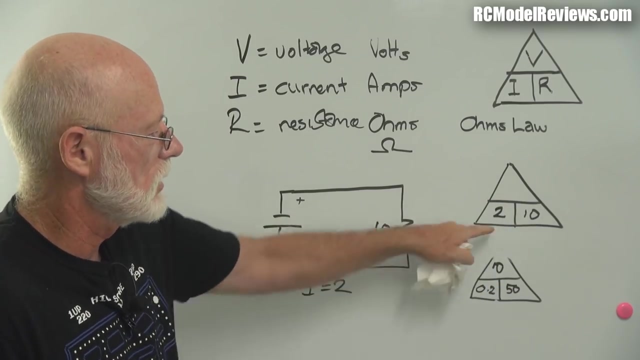 i need more space on the board. here we go. here's our ohms law triangle. this time we know the resistance, that's 10, and we know the current, that's two. now, because these are on the same line, we multiply them together to get the missing value, so it's 2 times 10. 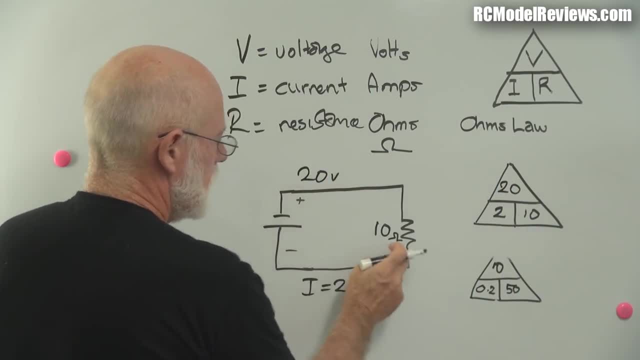 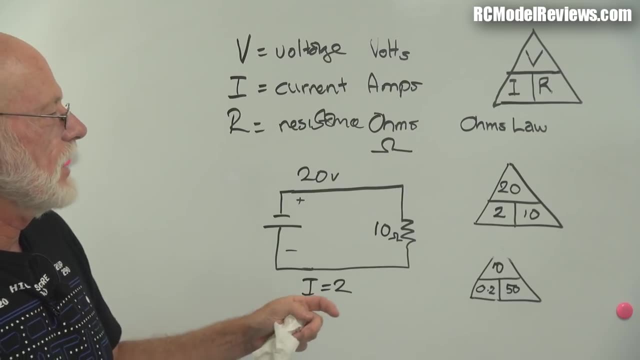 20. so we need 20 volts to get a current of 2 amps through our 10 ohm resistor. it's all it all comes together. math's really simple and even if you don't know how to rearrange algebraic formulas, then you can use this triangle and you can calculate all that stuff out, because 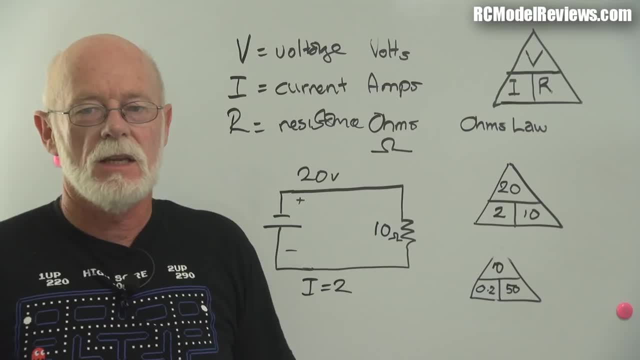 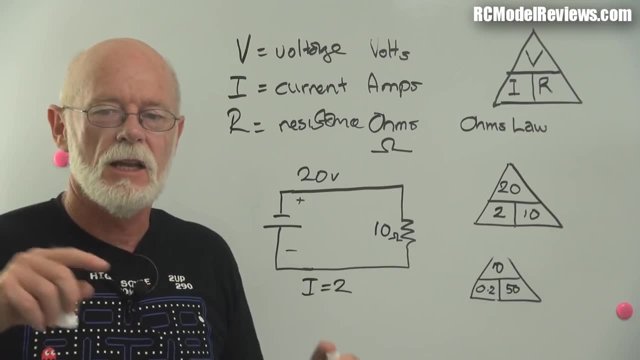 we're going to use this ohms law triangle because in the next video i'm going to calculate the internal resistance of a lipo battery and show you how you can do it yourself if you wanted to, although most charges have got a little facility now you press buttons and 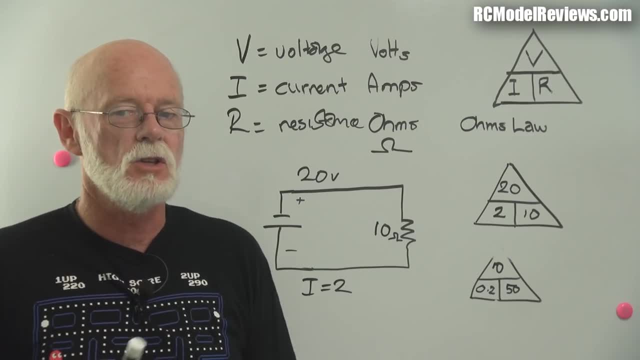 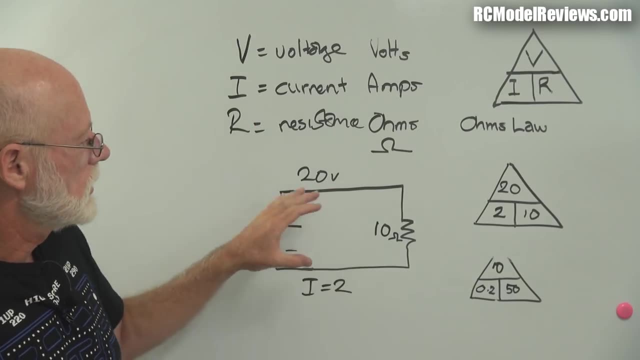 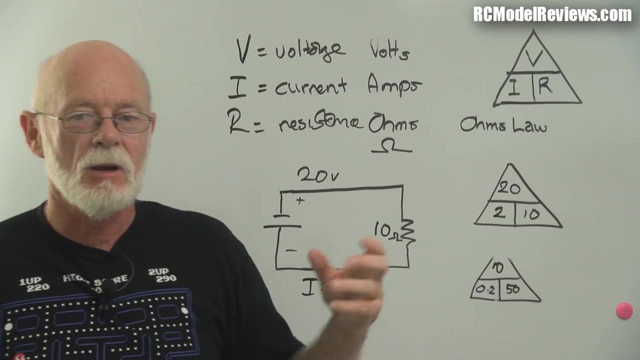 it'll show you the internal resistance. it's not always accurate, because internal resistance of batteries can vary depending on a number of things: temperature and also the current you're drawing from it. when you draw tiny little amounts of current from a battery, the internal resistance appears to be much lower than when you draw large amounts of current. so depending on how much, 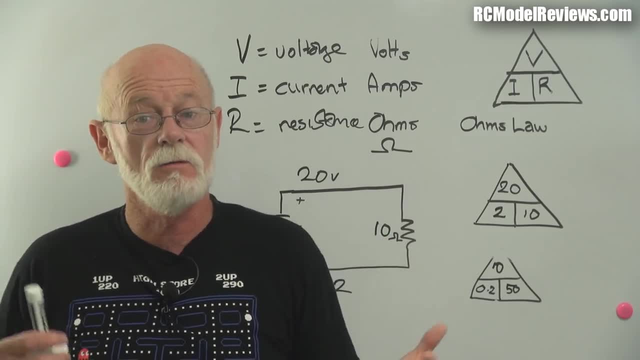 current you use to do the test, the internal resistance result you get will vary significantly, and i'll show you that in the next video as well, because the figures i mentioned in the next video are going to be much lower than the ones that i've shown you in my previous videos. so keep watching. 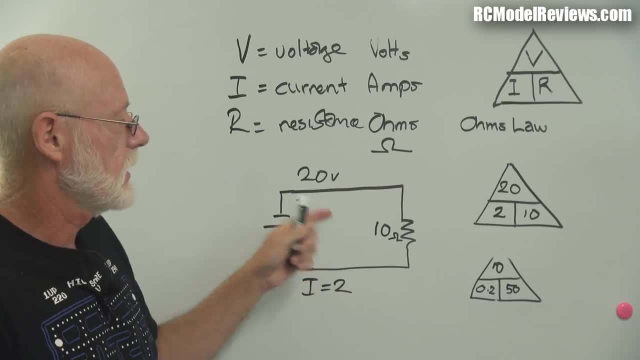 because the figures i'm going to show you guys are going to be bigger than the ones that i've seen in my previous videos. measured, we're at a much higher current than the figures the charger uses and I got quite different results to the numbers the charger produces. but also 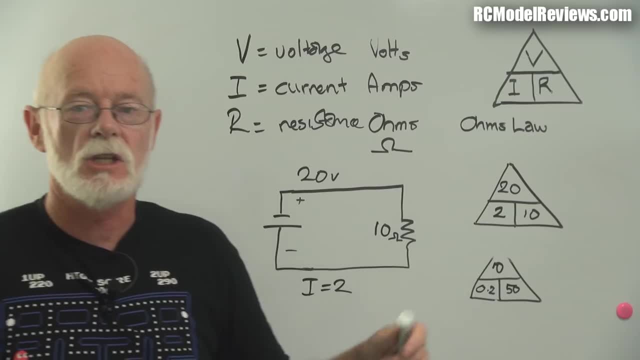 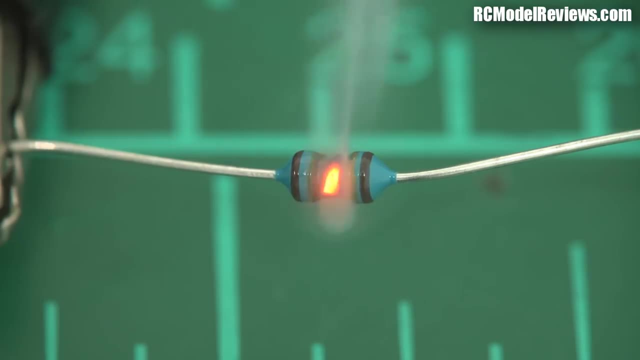 what I'm going to do is show you now about power, because we've got voltage current resistance. but ultimately, if we do this, if we put a current of two amps through a 10 ohm resistor, it's going to get hot. I mean resistors get hot when. 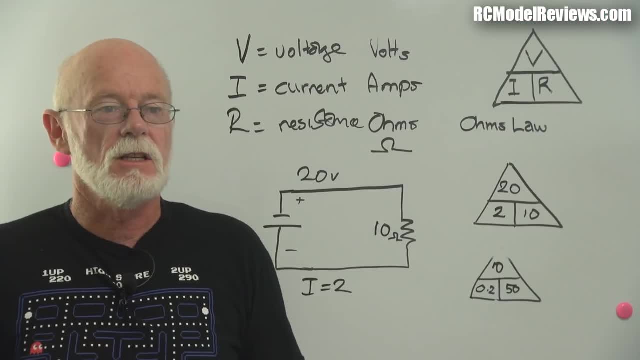 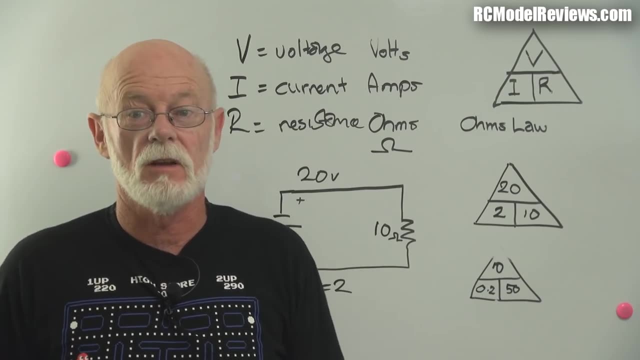 you put current through them. that's what happens, because electricity is of no use if it doesn't do any work. I mean electricity. if electricity flows and this it causes something to happen, well, there's no point in having it flowing. so this is sort of the equivalent of a a bar heater in a resistive heater, if you. 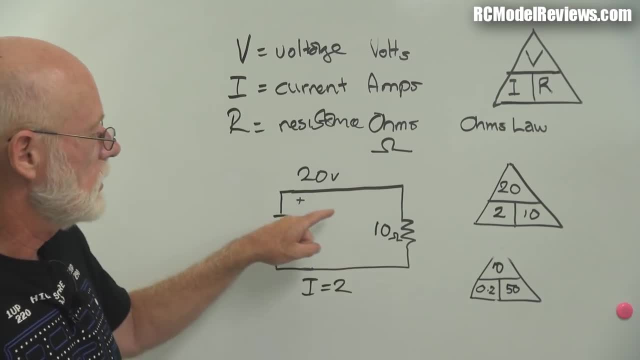 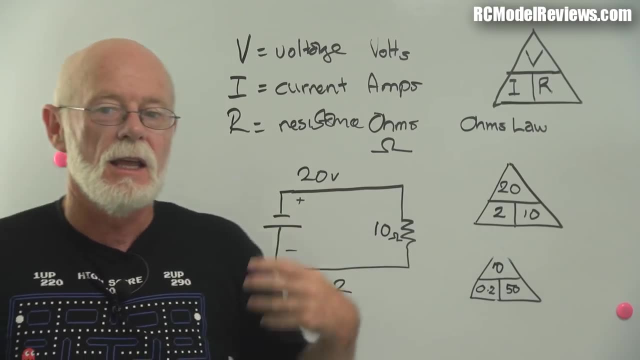 got a heater in your living room where you might use an electric jug or any of those things. what we do is we pass a current through a resistor and, in the process of squeezing through that resistor, as this resists the flow of electricity, it creates heat, and that's where we turn our electricity into. 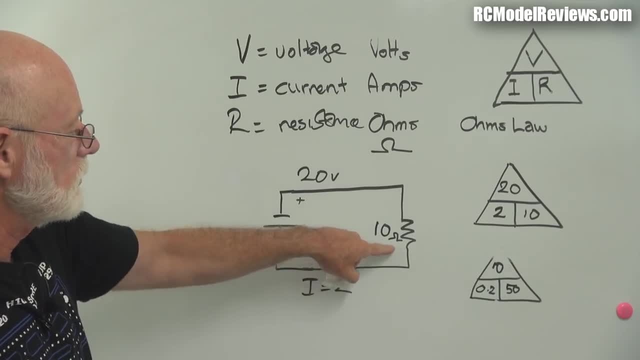 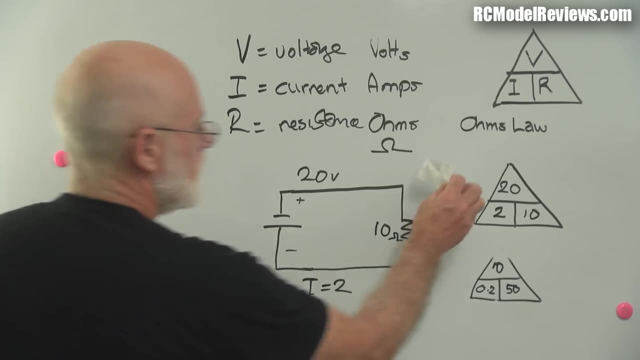 something useful. it turns it into heat. so how much heat would we get from, or how much power would go into, this 10 ohm resistor? how can we calculate that? well, you know it's, it's. it's a lot of work, but you need a lot of fun. let's go over here. 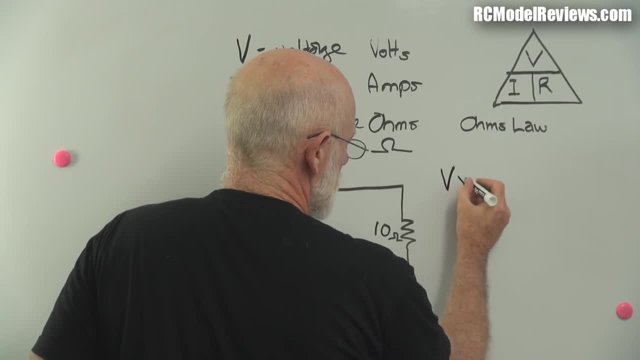 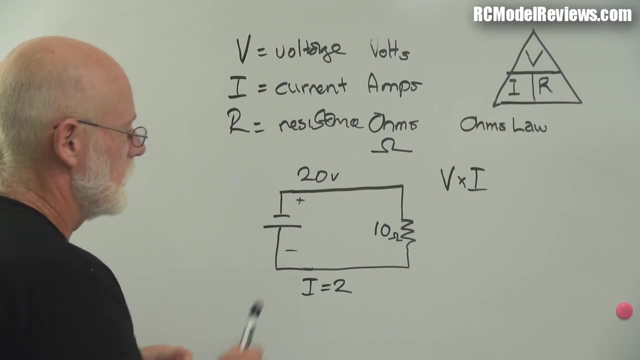 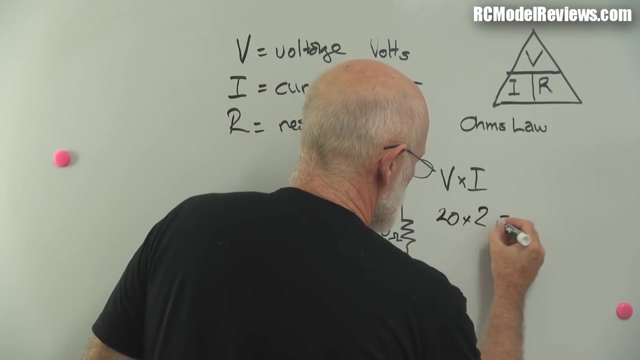 I'll do a formula for power power formulas really easy. it is the voltage times the current. there we go. so if you know the voltage, you know the current, you can calculate the amount of power that's going to be produced. so in this case, yeah, we know, we've got 20 volts times the current is 2 amps, so we're. 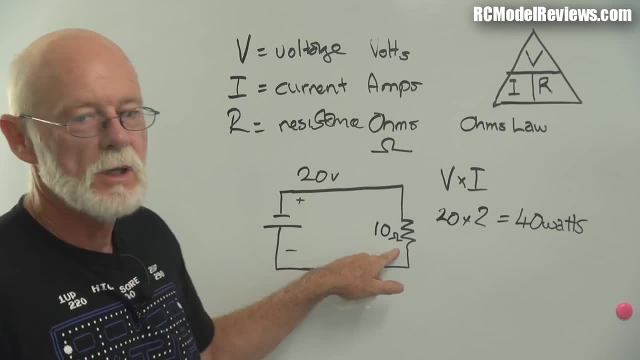 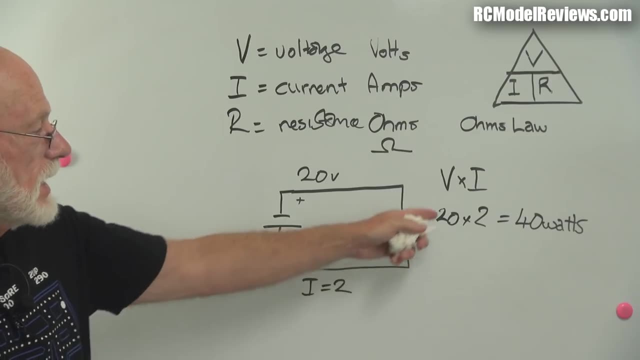 going to get 40 watts. what's this? how we measure our power? so this resistor here here would have 40 watts of power being dumped into it, So naturally it would get hot, because 40 watts is quite a bit Simple, easy peasy, lemon squeezy. So that's how we can calculate. 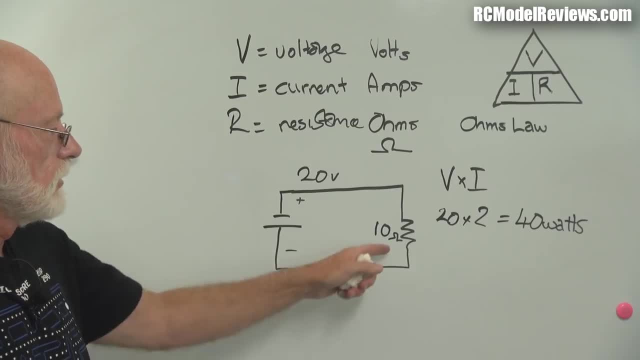 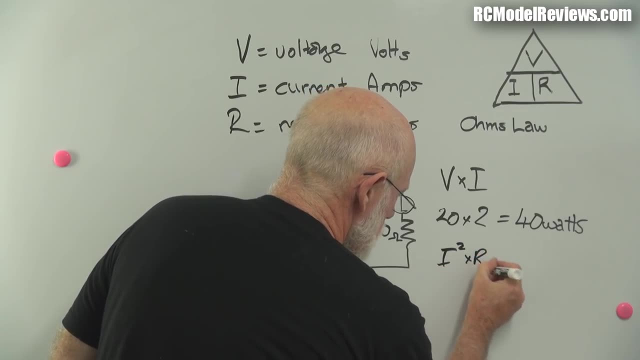 the amount of power going into our resistor. But there's another formula too we could use, and that is I. that's the current squared times the resistance, And so we know those figures. Let's see if that produces the same thing. Now the current is 2,, 2 amps, So let's. 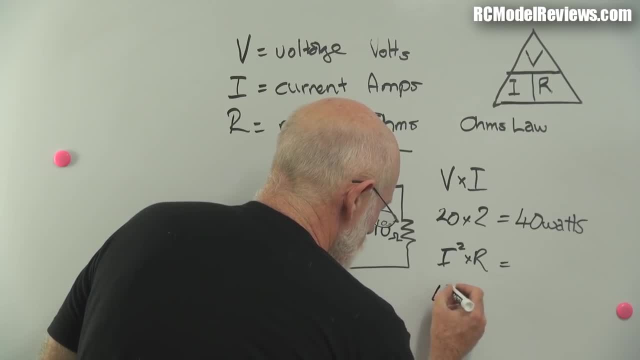 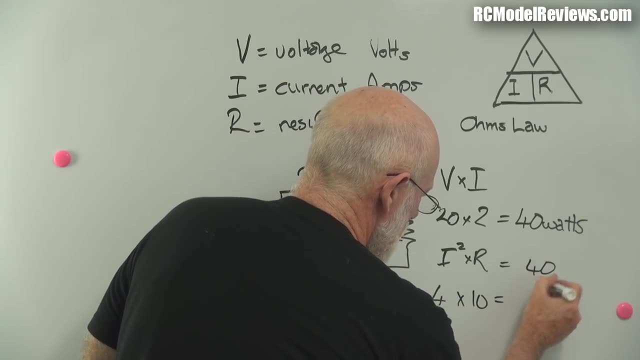 say 4, because that's 2 times 2. squared is 4, 2 times 2 is 4.. Multiply that by the resistance, which is 10 ohms, And that also equals. this, equals 40, and so does this. Oh, sorry that. 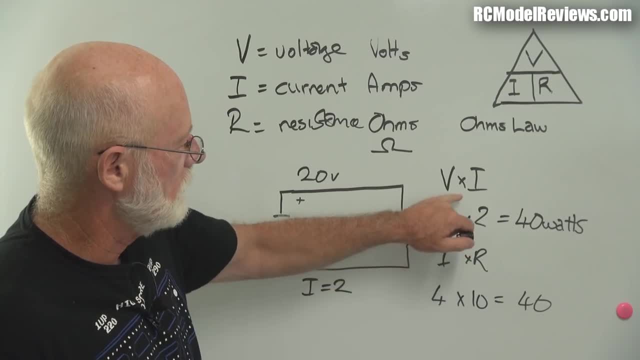 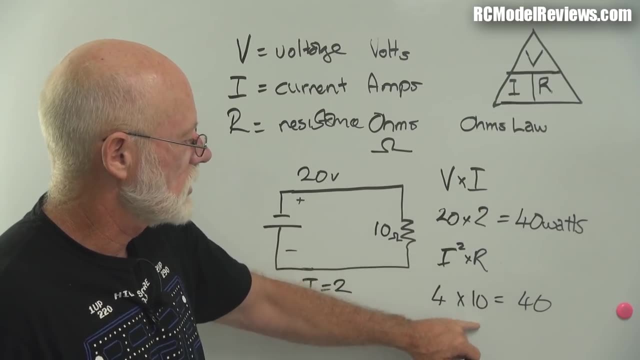 doesn't? that's just symbolic. So yeah, so we get the same result. whether we use this formula: V times I or I squared times R, Whether we multiply the voltage by the current or we square the current and multiply by the resistance, We still get the same figure of. 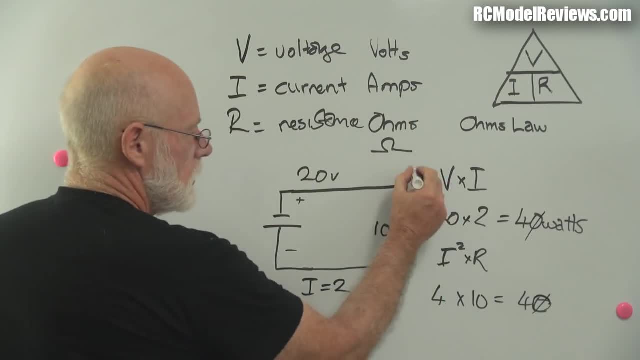 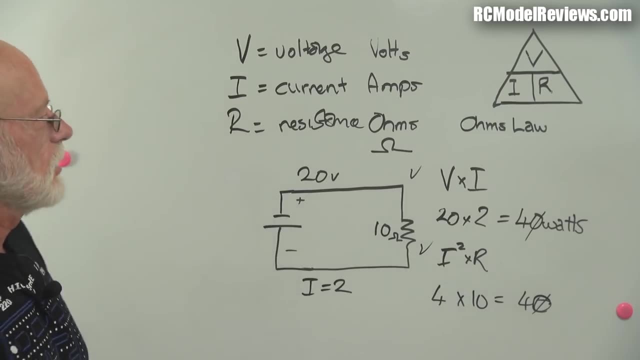 40 watts But now. so we have two formulas here that we will use. We will remember for later on when we look at batteries and power and things like that. So it's Ohm's Law, It's really, it's really simple. It might look complicated because 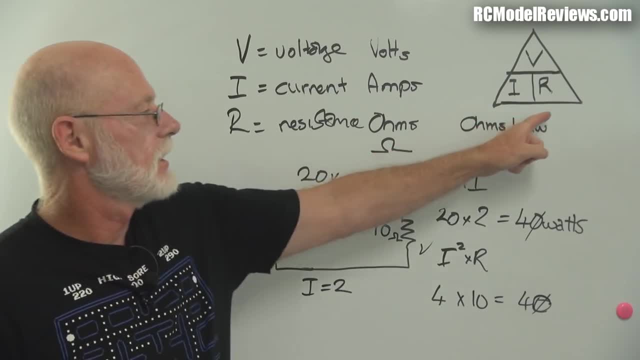 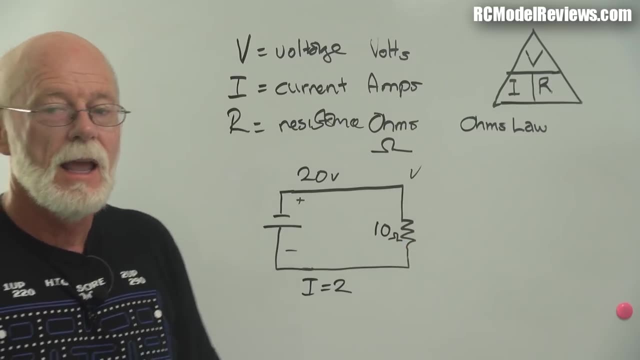 of the algebra involved and the formulas. But honestly, this little triangle here makes it simple And, as you can see, if we know this stuff we can work at some really cool things. There we go: basic Ohm's Law. This will come in handy when I do my ham radio. 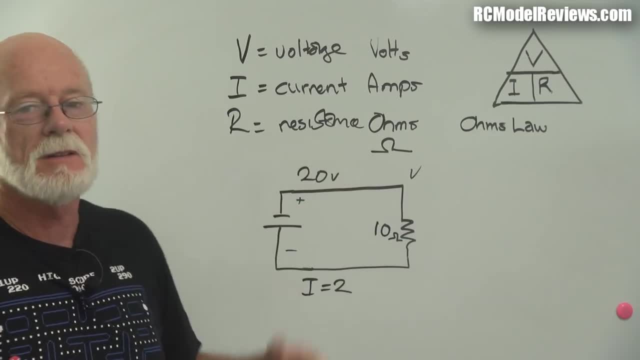 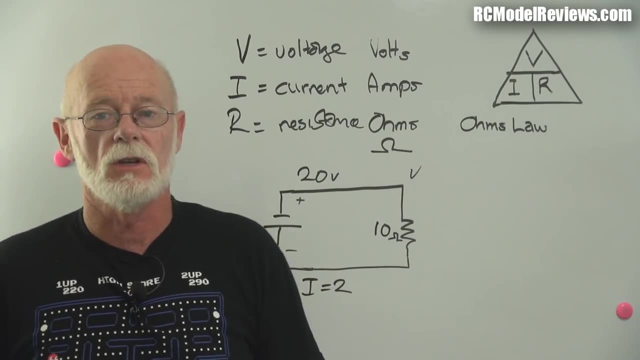 series as well, because this is one of the basic fundamentals of electronics and electricity. If you don't know this, then there's no good learning other stuff, because a lot of stuff is based on this. You need to know how electricity flows Through a circuit to understand more complicated concepts. So there you go. That's Ohm's Law. 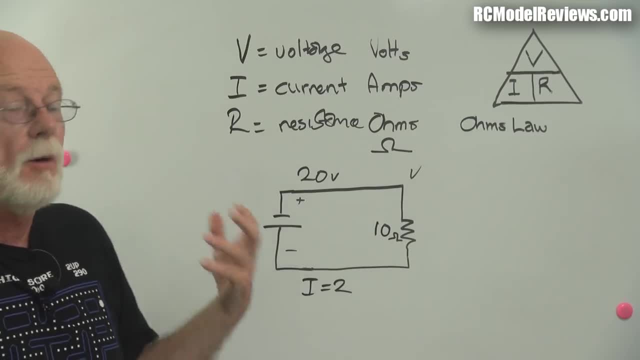 If anyone's got any questions about this, then put them in the comment section. If you've got any comments, put them there as well, because that's why it's called the comment section, and I'll do my best to address your comments and your questions.